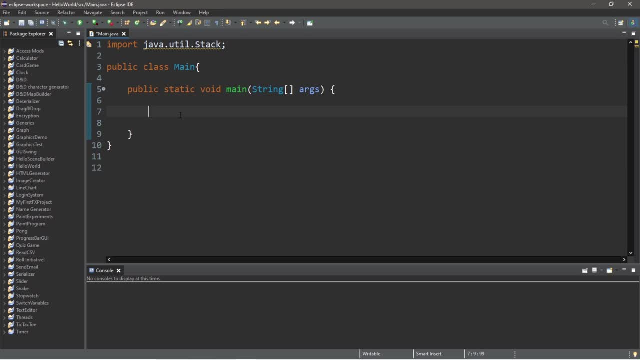 so i'll stick with that. now, to push objects onto our stack, we first need to declare our stack and instantiate it. so let's do that stack, then we will list the data type of the objects that we will be adding to our stack. so the launched objects let's select, except for we have the. 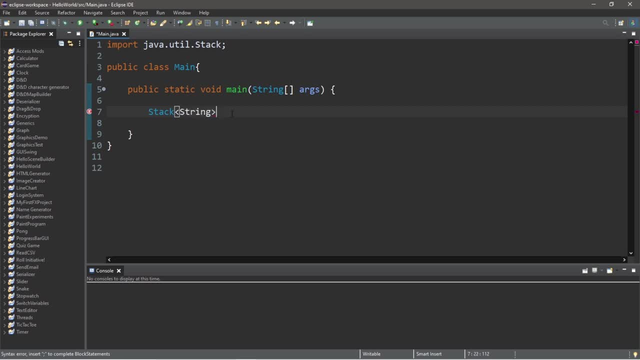 first stack and then we'll hide all of the objects that were added. let's take the numbers. Luckily, strings are a type of object and they're fairly simple, so we will create a stack that can store strings: the names of video games. 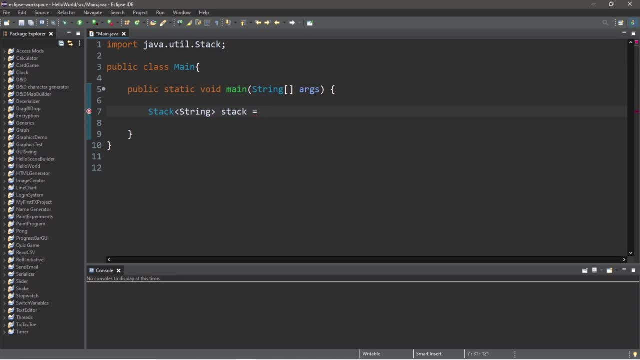 And I will name the stack stack to keep it simple. Stack stack equals new stack, And I will list the data type and then add a constructor. Okay, so we now have a stack data structure. Now, with stacks, they have five unique methods. 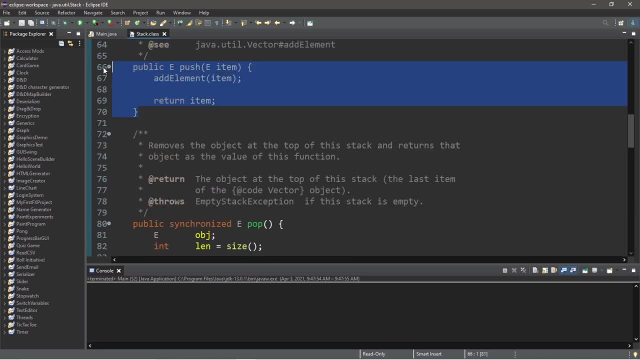 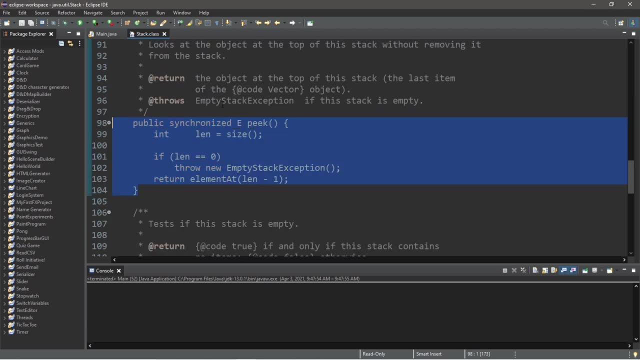 Let's take a look Now with stacks. we can push an item onto the top of our stack. We can pop an item from the top of the stack. We can peek at the item at the top of the stack. We can check to see if our stack is empty. 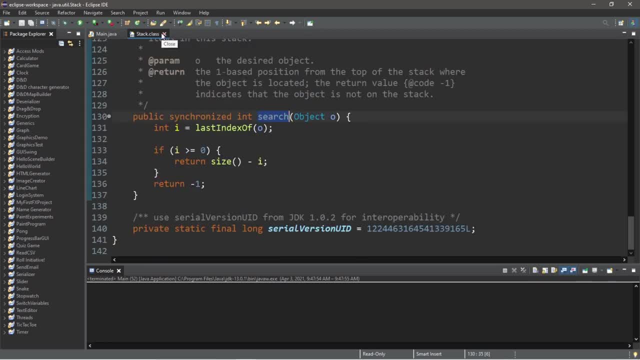 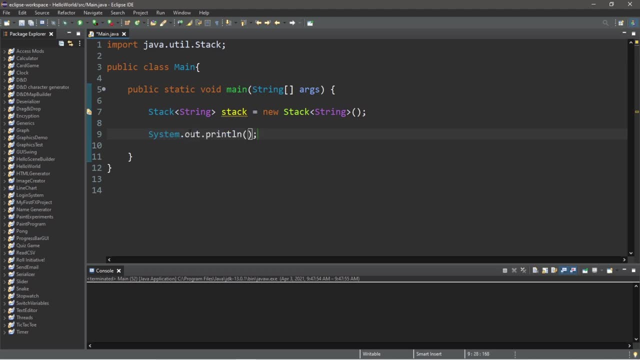 And we can search our stack for an item. So those are five unique methods available to stacks. Let's first check to see if our stack is empty. So let's use systemoutprintln. And currently our stack is empty. That is true, but that'll change soon. 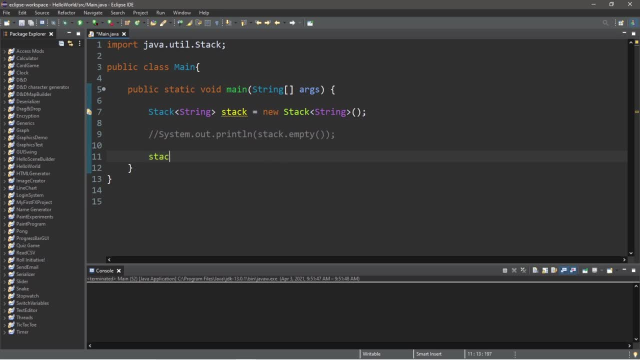 So let's push some games onto the top of our stack. So we type the name of our stack, stack and use the push method, Then pass in our object. So we will pass in a string the name of a video game. 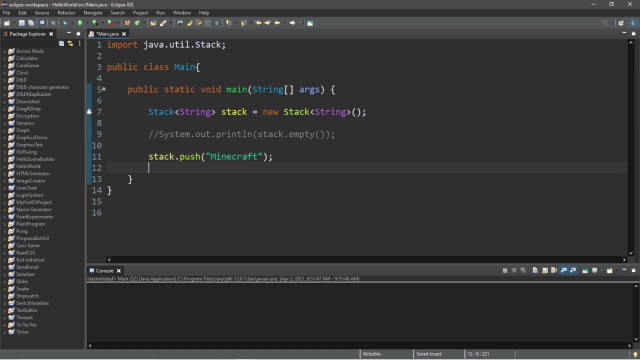 Let's add Minecraft first, Then let's add Skyrim, Then Doom. You can pick your own games if you want, I don't care. Then Borderlands And then Final Fantasy VII, FFVII. Okay, let's check to see if our stack is empty now. 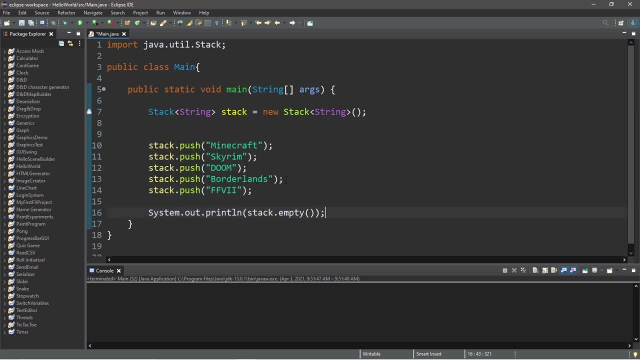 So let's move this line of code to the bottom And run it, So our stack is no longer empty. This returns false. So with a stack we can at least take a look at the items within the stack without removing them. So let's use systemoutprintln and I will print my stack. 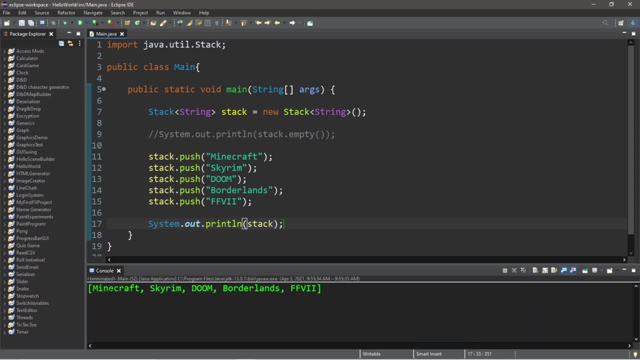 So this will print all of the objects within my stack, beginning with Minecraft, then Skyrim, Doom, Borderlands and Final Fantasy VII. However, by printing our stack, we're not removing items from the stack, so that's completely fine. 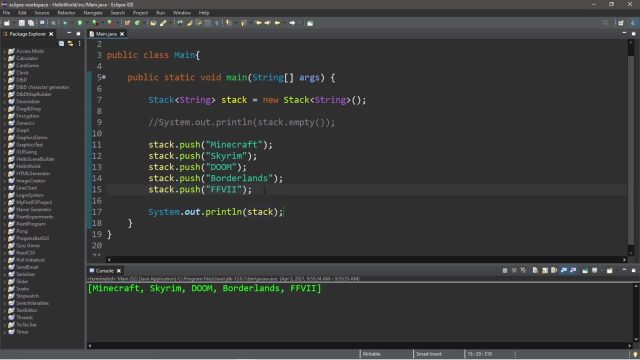 So this time let's pop the topmost item from our stack by using the pop method, stackpop, And we don't need to list an object, because pop will always remove the topmost object from our stack. So now Final Fantasy will be missing from the top of our stack. 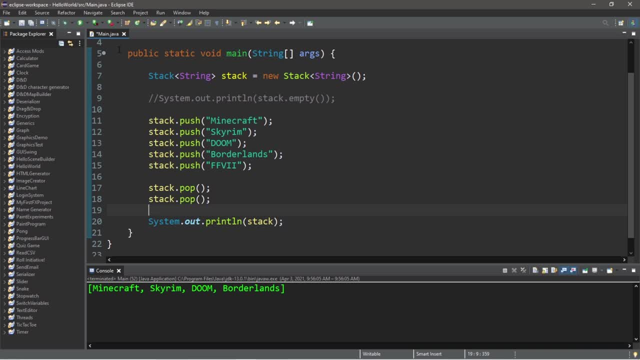 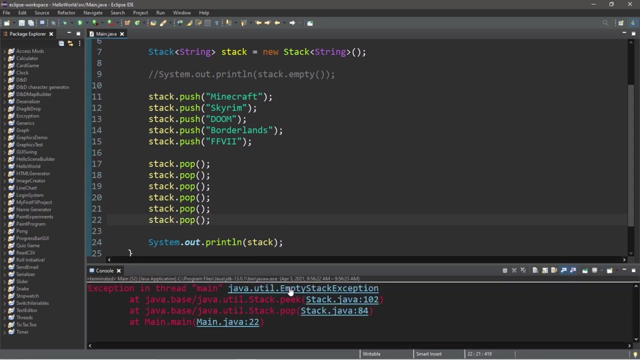 So if I was to repeat this again, well then this will remove Borderlands, And then Doom, Then Skyrim And then, lastly, Minecraft. Then if you pop again, this is what happens: An exception, Empty stack, exception. So that's something to keep in mind. 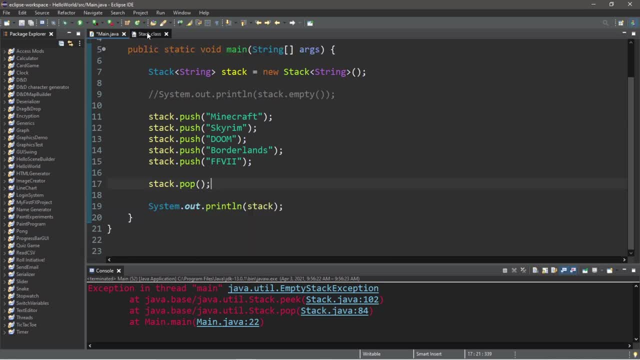 Now, when you pop the topmost object from a stack, this will actually return that object. If you need the object from the top of the stack, you can pop it and then assign it to something. So let's say string myfavegame equals stackpop. 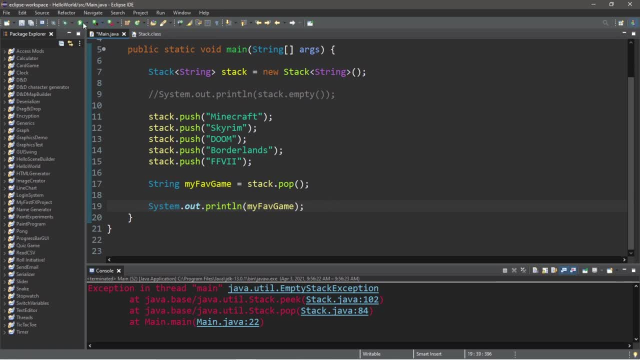 And then I will print myfavegame And this will print Final Fantasy VII And it should be missing from the top of my stack if I was to print my stack. So Final Fantasy VII is no longer in my stack Because I popped it, then assigned it to the string variable of myfavegame. 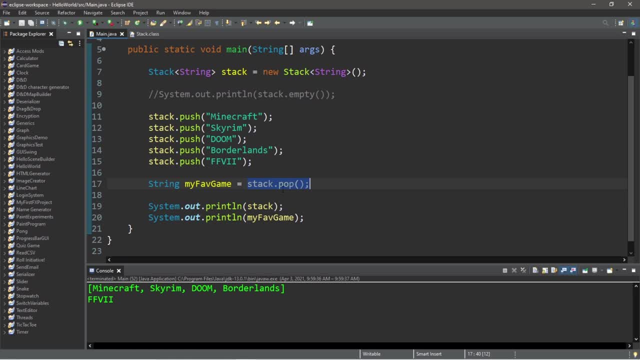 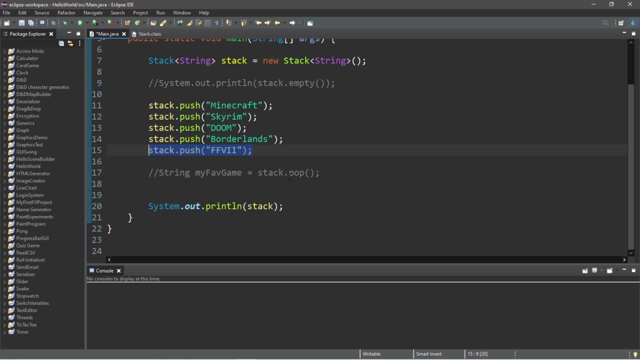 So, in order to take the topmost object from a stack, you use pop and then assign it to something. If you ever need to take a look at what the topmost object is within your stack, you do not want to use pop, because that will remove it. 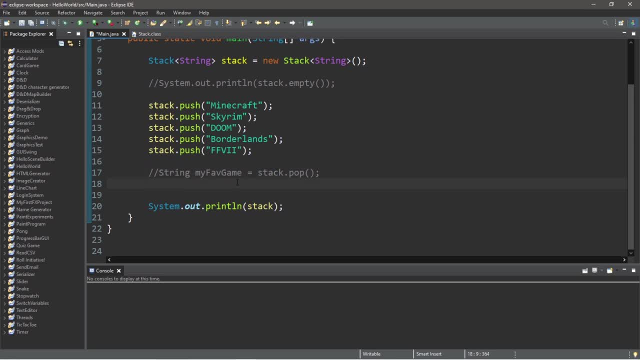 You can instead use the peek method of stacks. So what I'll do is systemoutprintln stackpeek And then immediately follow this with printing my stack. So let's run this. So the topmost item within my stack after using the peek method is Final Fantasy VII. 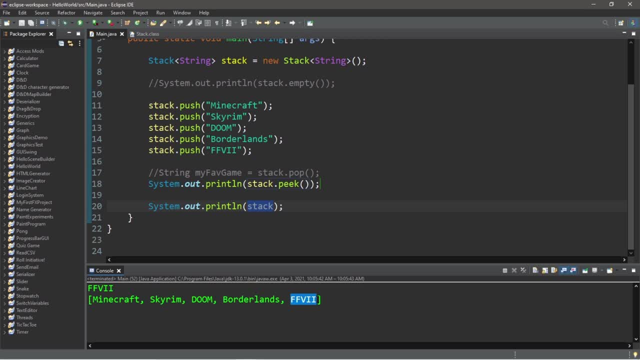 Then, after printing my stack, Final Fantasy VII is still at the top of my stack. So if you ever need to take a look at the object that is at the top of the stack without removing it, you can simply use the peek method. 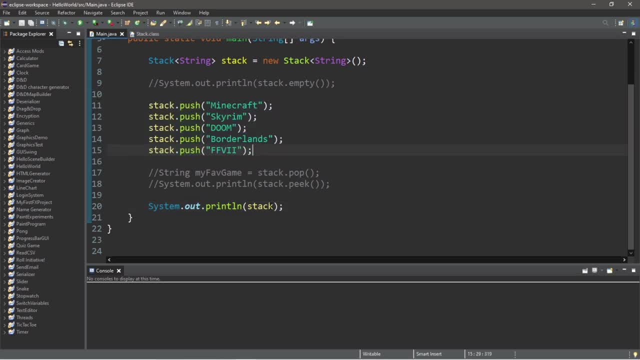 If you need to search for an object within the stack, you can use the search method. Let's print stacksearch And we pass in our stacksearchsearch And we pass in our object as an argument. So the very first item in a stack will have a position of 1.. 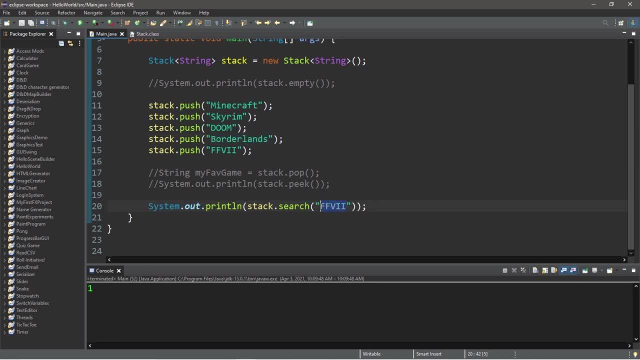 You would think it's 0, but it's actually 1.. Now let's find Borderlands. That will be in position 2 from the top, Then Doom would be, of course, 3.. Skyrim is 4.. Then Minecraft is 5.. 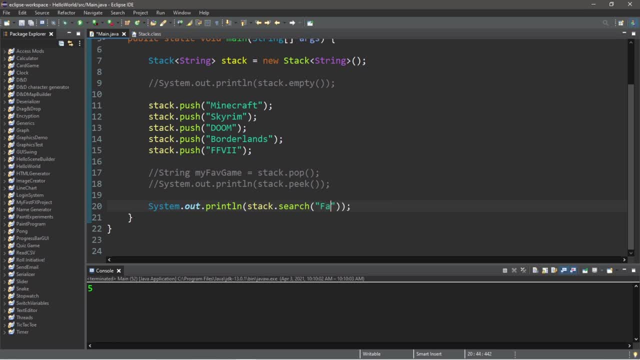 So if you search for an item that is not within the stack, like Fallout 76,, well then, this will return negative 1.. Well then, this will return negative 1.. If search does not find this object within your stack, it will return negative 1.. 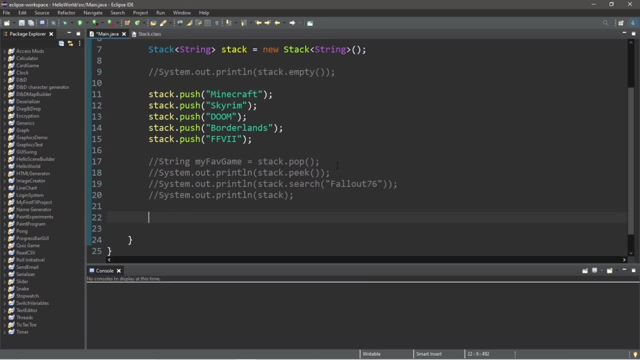 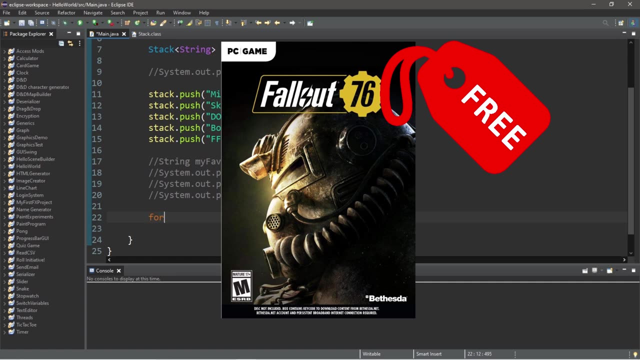 So with stacks we can actually run out of memory. So let's add like a billion copies of Fallout 76. We find Bethesda's warehouse of unsold Fallout 76 games, So we'll create a stack of a billion copies of Fallout 76.. 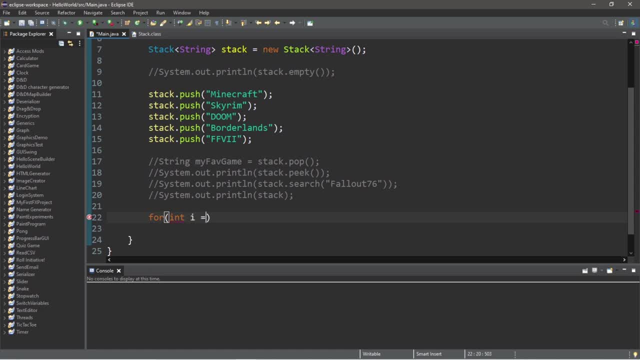 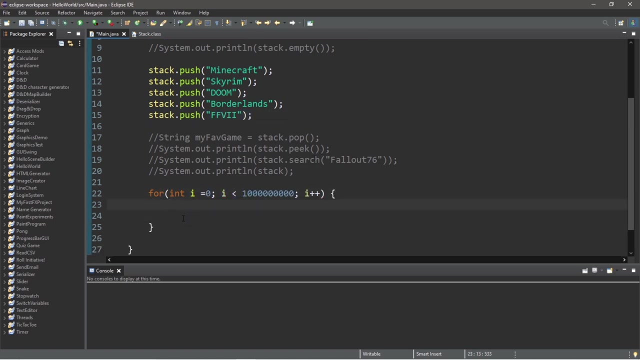 We can do this using a for loop. int i equals 0, as long as i is less than like 1 billion, That's probably close enough. increment i. Then we will push a copy of Fallout 76 to our stack. So stackpush fallout 76.. 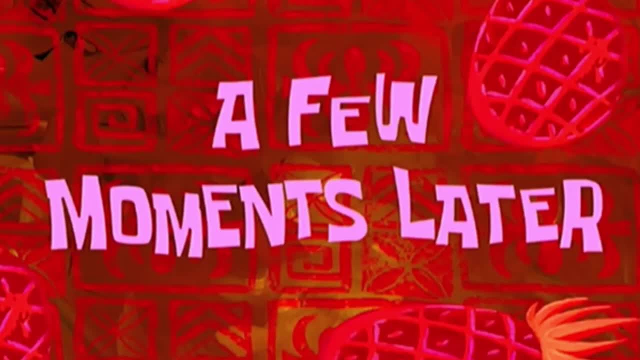 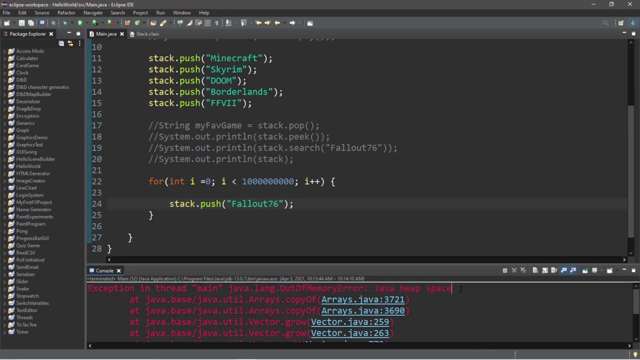 And this is what happens A few moments later. So we will run into an out of memory error due to the Java heap space. So it is possible to run out of memory when adding objects to our stack. Now this is an interesting feature that may or may not happen to you. 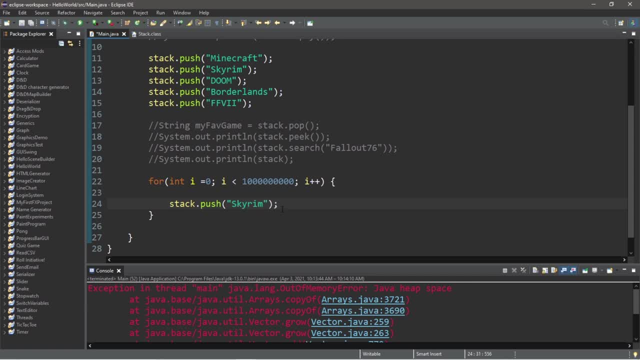 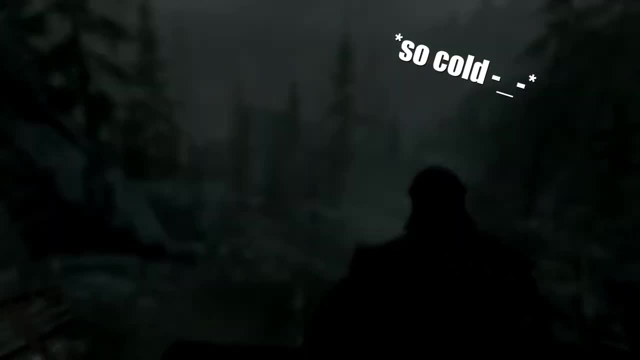 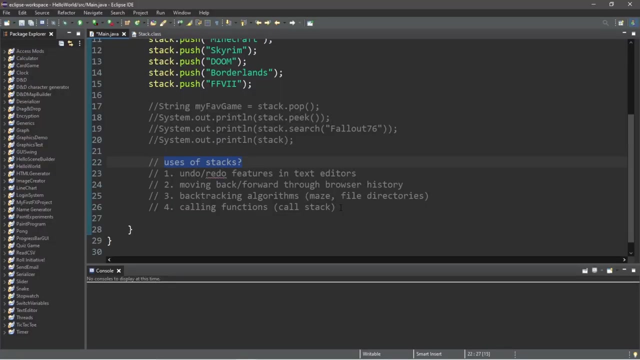 If you add a billion copies of Skyrim onto a stack. Dammit Todd Howard, you did it again. Now what are some uses of stacks? Here's a few examples. One: we can use them in undo redo features in text editors.